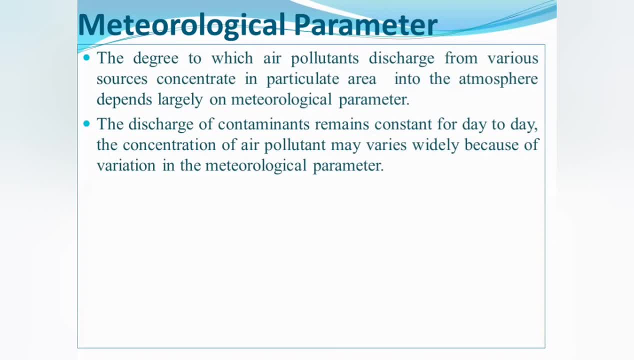 The concentration of air pollutant may vary widely because of the variation in the metrological parameters. The discharge of particulate matter depends on how the metrological parameters vary. For example, if the variation of temperature goes to higher altitude, it will decrease. 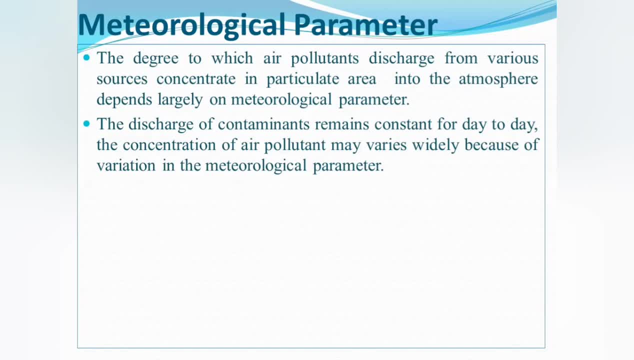 If it goes to higher altitude it will decrease. Actually it decreases. The dispersion of pollutants is also a criterion. We will see the environmental and adiabatic lab set in detail later. The dispersion of pollutants depends on the metrological parameters. 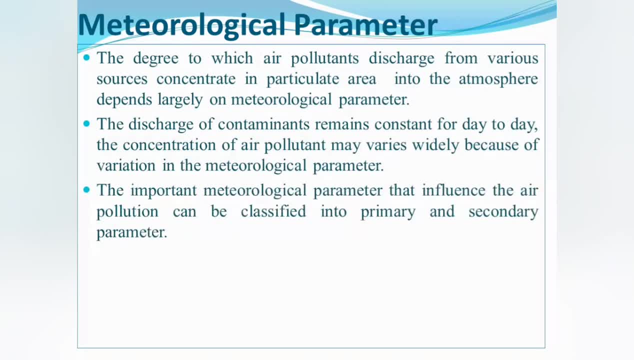 The important metrological parameters that influence the air pollution can be classified into primary and secondary parameters. The important parameters are primary and secondary. The important parameters are primary and secondary. The metrological parameters depend on the primary and secondary parameters. Due to the metrological parameters, the weather changes and climate changes depend on the metrological parameters. 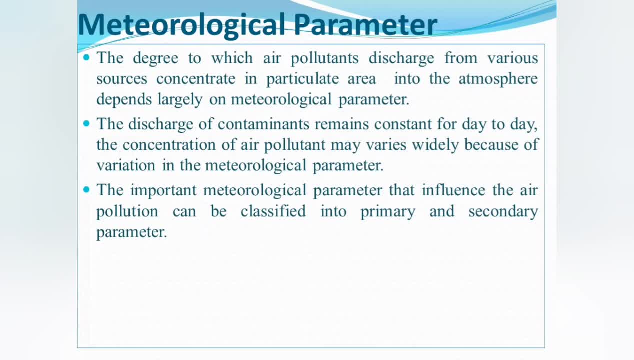 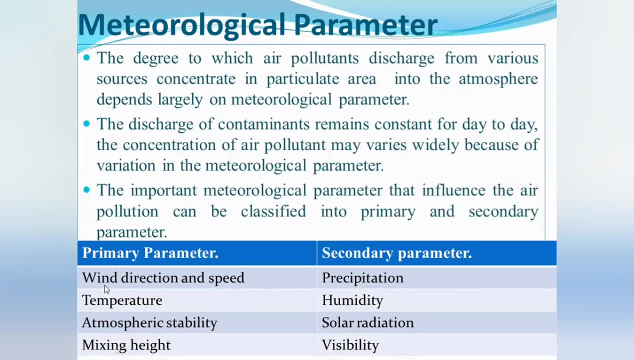 The metrology studies, the primary and secondary parameters. What are the primary and secondary parameters? The primary parameters are wind direction and wind speed, temperature, atmospheric stability. What are the primary and secondary parameters? There are a variety of types, like stable發, decreased temperature, mild temperature. 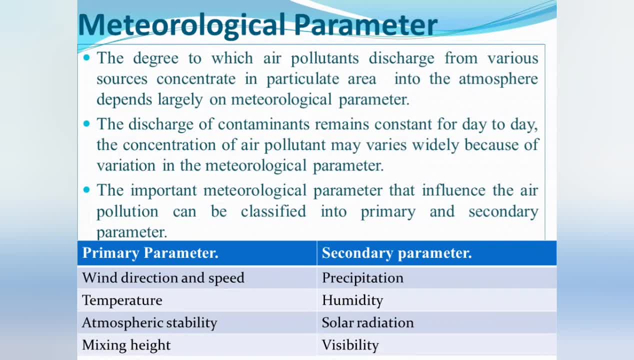 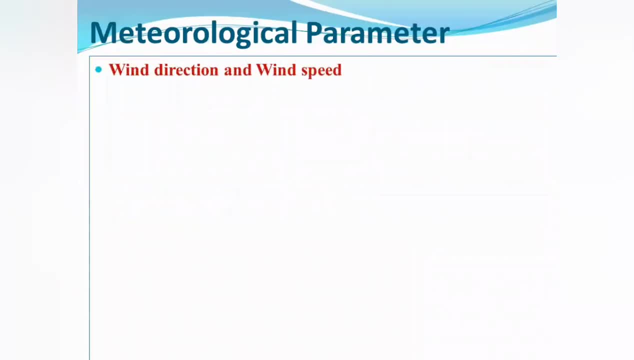 Balanced temperature and calent atmosphere. we will see primary parameters in detail in next video. we will see secondary parameters in detail. So wind direction and wind speed is first. The dispersion and diffusion of air pollutant depends on wind direction and wind speed. With high wind, current pollutants 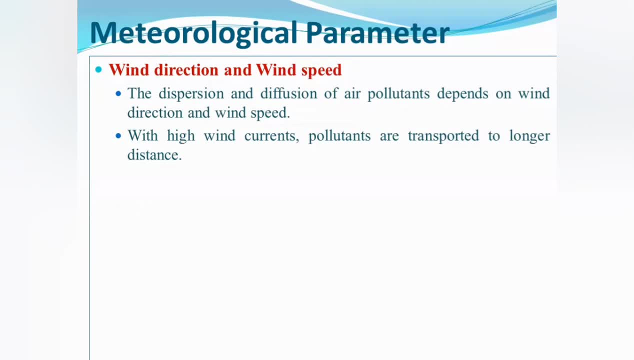 are transported to longer distance. If pollutants are emitting from industry or from solid waste disposal site, the dispersion of pollutants will remain near the source or away from the source. Source means where pollutants are emitting, So it totally depends on wind direction and wind speed. If wind speed is high, pollutants will travel to longer distance, Longer distance. 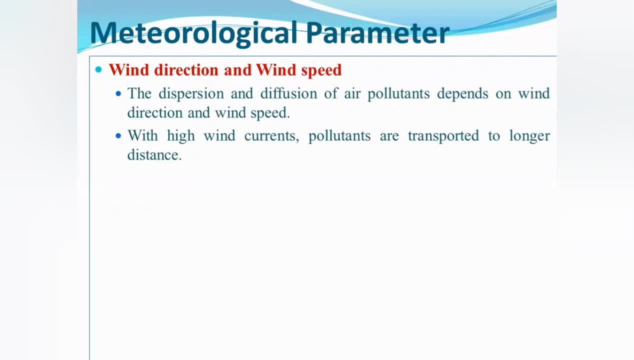 travel means they will be dispersed. Their concentration will be like this, So the dispersion of air pollutant will be too much, So its more visible from distance. In this video I show how the air pollutants are. transportation- the dispersion of air pollutants in the system. 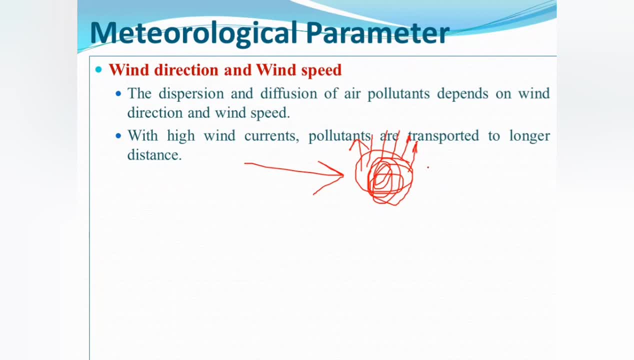 and annoyed airotics in the system. In next video I show how. tell you which is Typhoon 4 & god Körper'sabe, fire mode Only sensor used in this video. Yes, Yes, Yes. So what will happen is that all pollutants will accumulate here, only around the source. 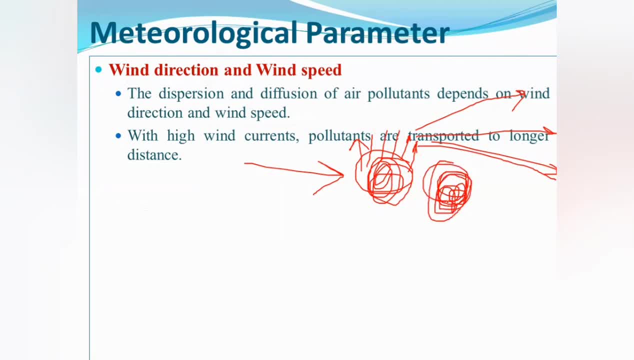 So if it accumulates around the source, then the concentration of pollutants will increase around the source. That's why it will be in a harmful condition. What we have to do, as much as possible, is that the pollutants have to be dispersed at a larger distance. 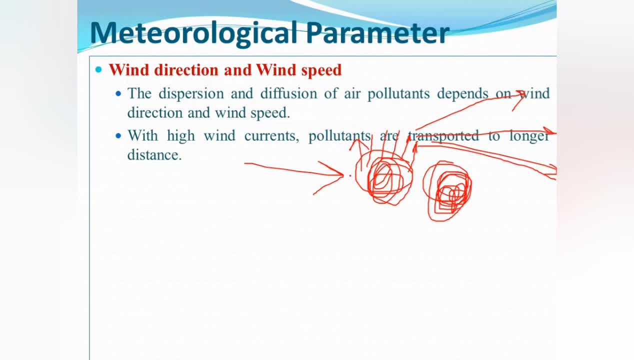 That's why wind direction and wind speed matter. Now I have told you about wind speed. What is the direction of wind? Suppose this is the source and the direction of wind is this: This is the source of air pollution. Suppose there are cities here. 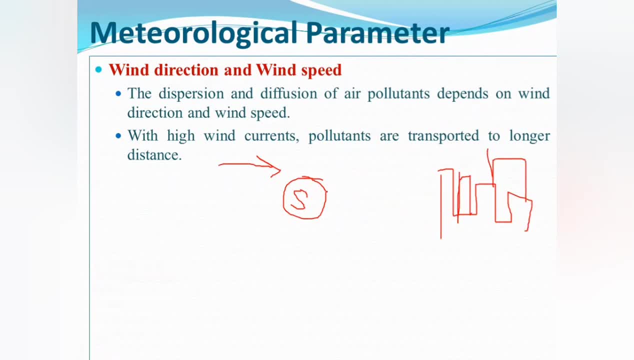 So all pollutants generated from the source will go towards the city, Towards the city, Towards the city. That's why this is the situation. Actually, the pollutants are dispersing here. The concentration will be less, But all the pollutants will go towards the city. 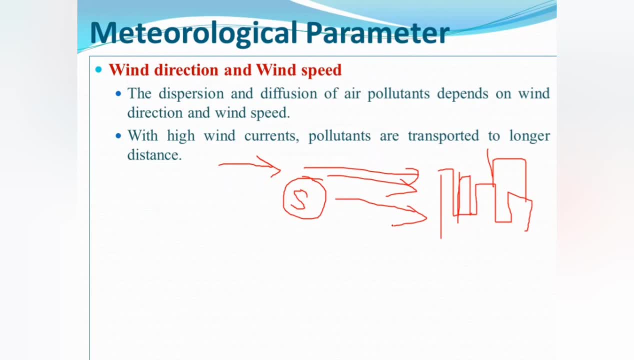 They will come towards us. That's why, while designing or planning the town, we have to keep all these things in mind. Wind direction, wind speed: What is the wind direction? In which direction does the wind stay for a long time? In which direction does the wind stay? 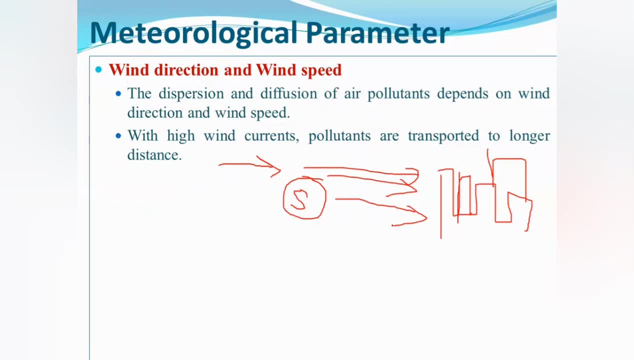 For example, conditions like this. So, for example, there is a lot of wind, So the wind is outside here, So temperature changes. When the temperature is high, the wind moves to the opposite direction. This is where the air is distributed at a larger distance. 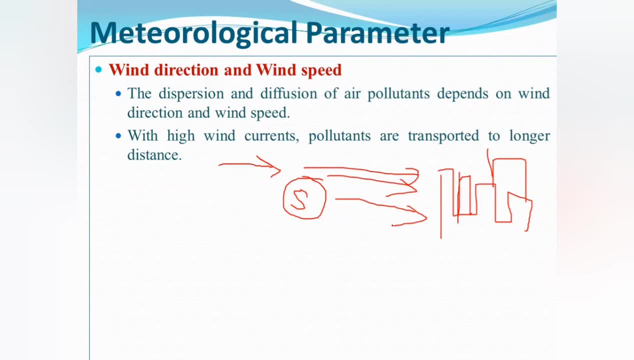 So in that case, the wind is not getting ionised. That is why there is a lot of wind, So the wind is not getting ionised. That is why the wind is not getting ionised, But the wind will not change because of this. 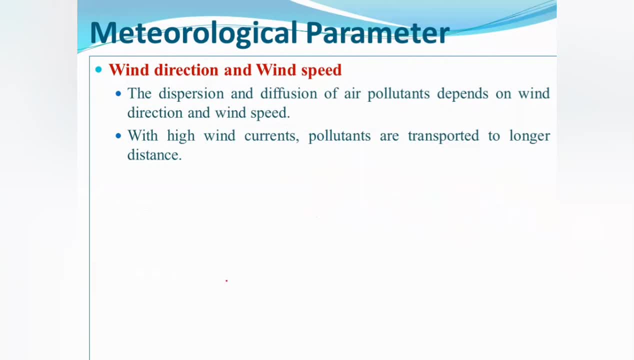 So it will be in any direction. We have to do it accordingly. We have to do it. All the sources of pollution mean the industrial area, So we have to allot in that way. 3. Next, temperature of temperature. 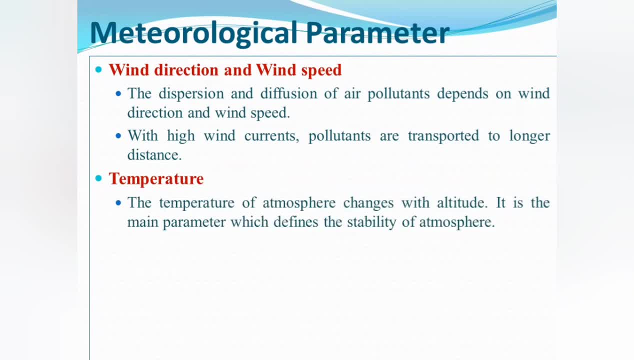 Let's see temperature metrological parameter parameter. The temperature of atmosphere changes with altitude. It is the main parameter which defines the stability of atmosphere. The next metrological parameter is mixing height. Mixing height is the height to which pollutant will extend into the atmosphere. 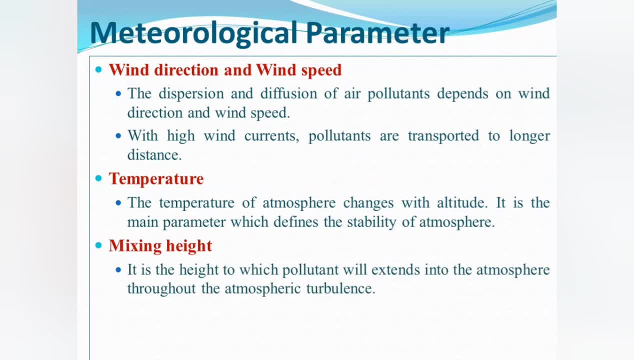 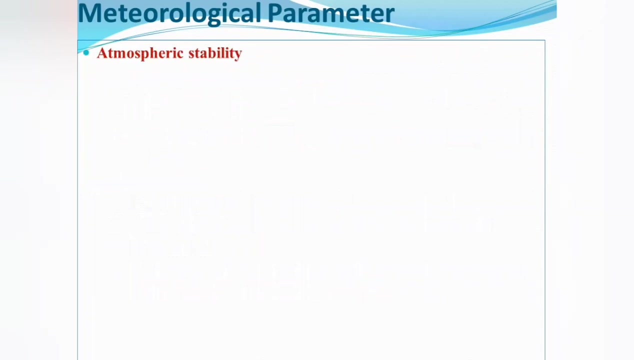 through atmospheric turbulence. Mixing height is the height to which pollutant will extend into the atmosphere through mixing height. Mixing height depends on atmospheric turbulence and wind speed. This is related to wind direction, wind speed and turbulence, Then Atmospheric stability. next was metrological parameter, Lucid. 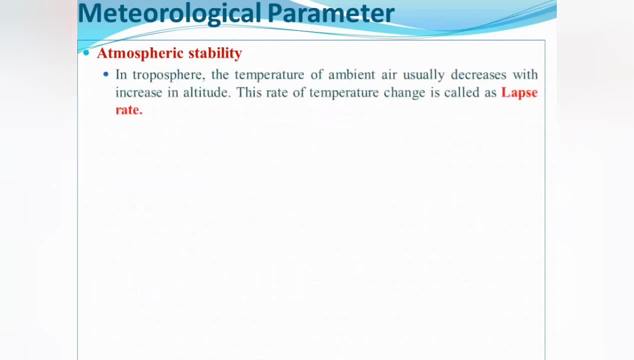 Moon maintain. in the tropical troposphere The atmospheric temperature of time, air and air STILES is usually decreases with increase in altitude. Aquí · – · · the temperature of the atmosphere decreases in the daytime. this rate of temperature changes is called as lapse rate, And this change in temperature with respect to altitude is called 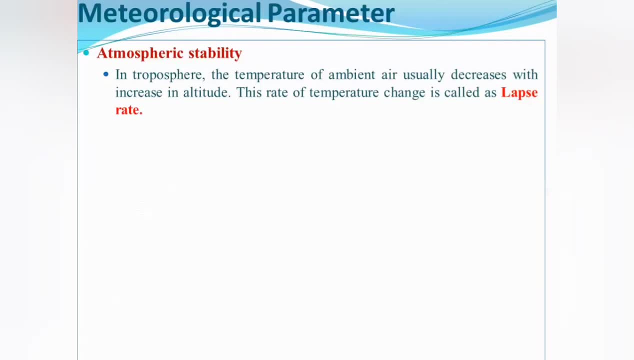 lapse rate. Now it is said that it usually decreases. Why does it decrease and how does it happen? I will tell you that. suppose, and it decreases in the daytime itself. Suppose it is earth. Now what is happening on it? Sun rays are coming from here, All ultraviolet. 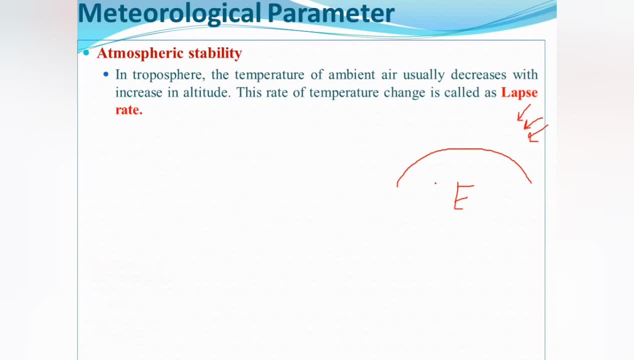 radiations of the sun are coming from here. So what is doing earth? What is doing earth? Earth is absorbing the sun rays coming from the ultraviolet radiation, Absorbing the heat. After absorbing the heat, it will emit the heat. What is the earth going to do? It will. 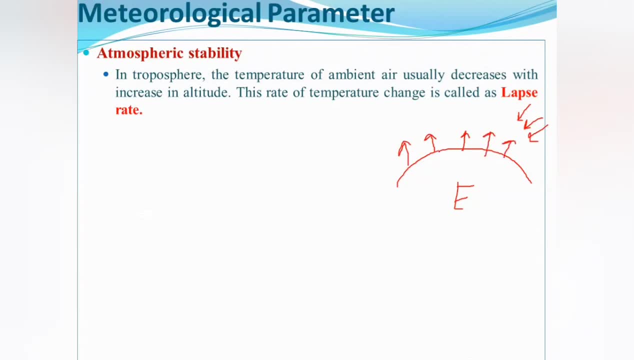 emit the heat. So when the heat will emit, then the atmosphere that will remain here, the atmosphere here, this atmosphere will be left at the same level. It will be left. Atmosphere is full of gasses. lower altitude gasses are more. lower altitude gasses are more, so heat will be absorbed more. 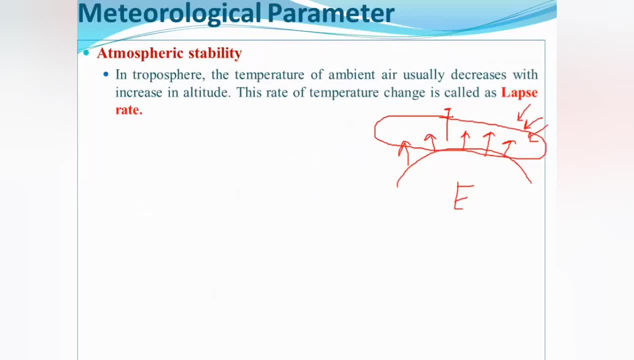 As we go upwards, the concentration of gasses will be less, like oxygen, nitrogen, what we have told you. their concentration will be less at higher altitude. Now, the concentration will be less at higher altitude, so the heat will be absorbed less, so the temperature will also be less. 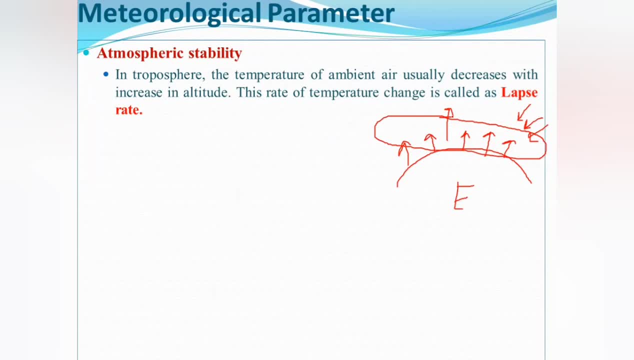 So this is the reason that what happens in daytime, as we say, in daytime, what does the earth do? It absorbs heat and releases heat. While releasing, the gasses present in the atmosphere absorb heat. because of that, only temperature variation occurs. Why in lower altitude there is more? why in higher altitude there is less temperature? the reason for that is that lower altitude gasses have less concentration. heat is absorbed less. 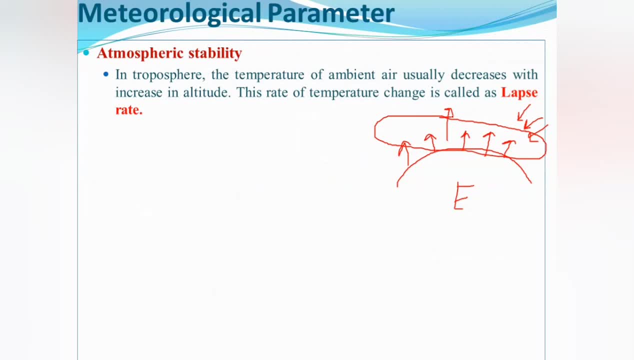 It's upside down again. gas concentration is less, heat is less absorbed and that is why the temperature is less. So this was the reason why it happens in daytime. Now I will tell you the inversion of night time. This rate of temperature change can be determined for a particular place at a particular time. 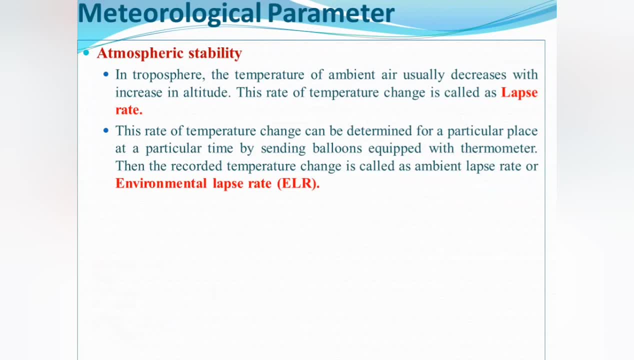 by sending balloons equipped with a thermometer To measure the temperature change. we have to fix the thermometer in the balloon and pass it at a higher altitude. As it goes at a higher altitude we have to check the temperature of the thermometer. Then the recorded temperature change is called as ambient lapse rate or environmental lapse rate. 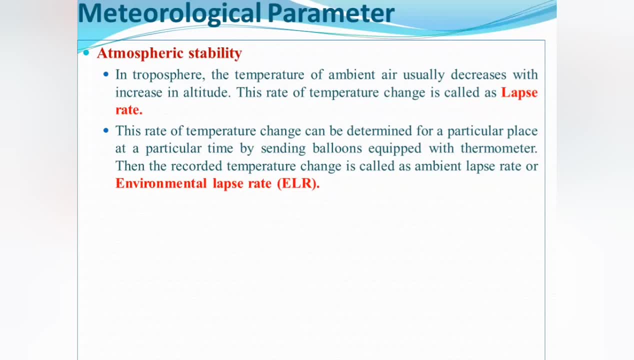 The temperature change that is going to happen is environmental lapse rate. It is a lapse rate, but why is it called environmental lapse rate? In the present condition, in the present time, the temperature change with respect to altitude. I am saying it again: in the present time, in the present area, in the present time, in the present area, in the present condition. 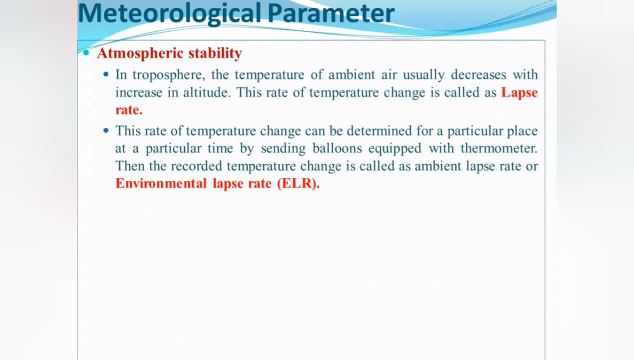 the temperature variation with respect to altitude is known as environmental lapse rate. Okay, This environmental lapse rate keeps changing, Because if the temperature variation in the afternoon will be different, it will be different in the evening, it will be different in the morning, it will be different in the night. 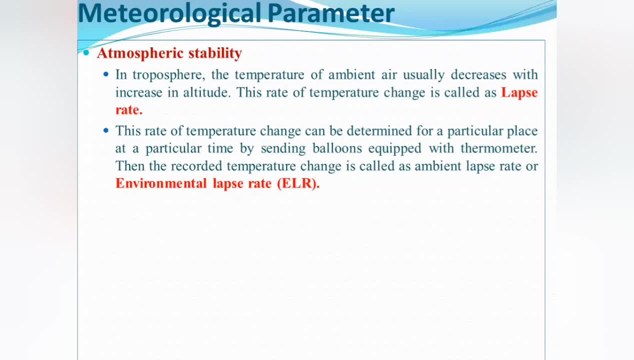 So that's why it is called environmental lapse rate The actual temperature lapse rate of the actual environment. the actual temperature change of the actual environment with respect to altitude, is known as environmental lapse rate. in simple terms, Then, environmental lapse rate changes from place to place, time to time, season to season. 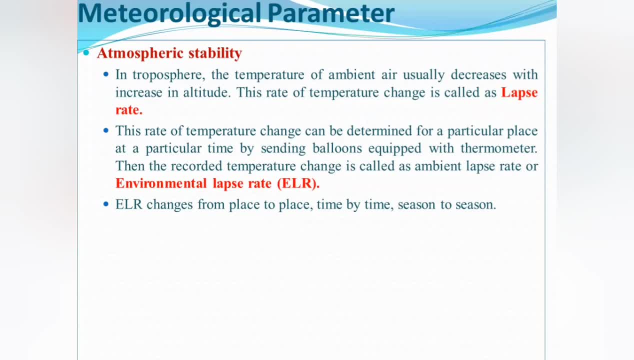 Environmental lapse rate means: suppose, after going up 1 km, if 5 degrees, suppose in today's time, if in winter, suppose in the afternoon- I am giving an example of 2 o'clock- that if we go up 1 km at a higher altitude, then if 5 degrees Celsius is decreasing, then in monsoon or in summer its rate will be different. 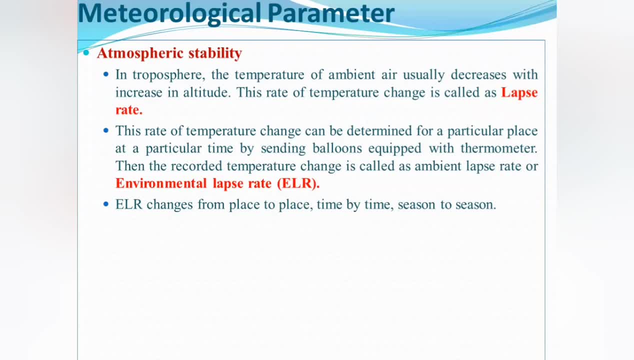 If we see that in the evening, then its rate will be different. That's why the environmental lapse rate changes from place to place, time to time, season to season. It will be different in Pune, it will be different in Mumbai, it will be different in Delhi, it will be different in Kolkata. 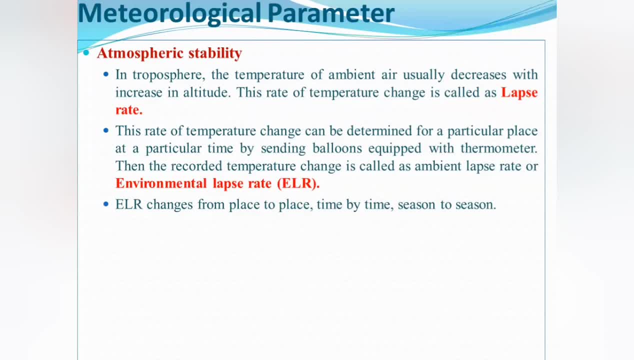 All these changes are different in environmental lapse rate. It is never constant. Okay, Then, when the column of hot air is released to atmosphere, it goes up in the atmosphere till its temperature becomes equal to the surrounding. How long does that air go up? 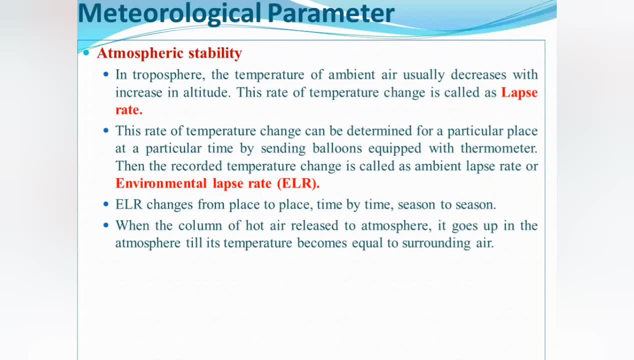 Until the temperature of that air is the same as the temperature of the surrounding. If it is the same, then the air, the parcel of air that we have sent, what happens to that air? then It becomes stable because the temperature of the atmosphere and the air that we have sent is the same. 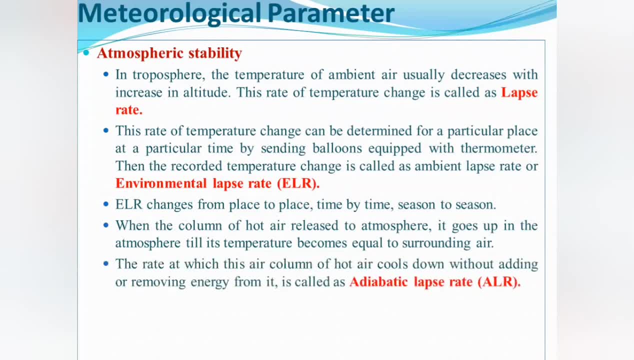 Okay, Then the rate at which this air column of hot air cools down without adding or removing energy from it. Okay, If, as I said, if we pass an air parcel in a balloon and fix the thermometer in it, Now what will happen? 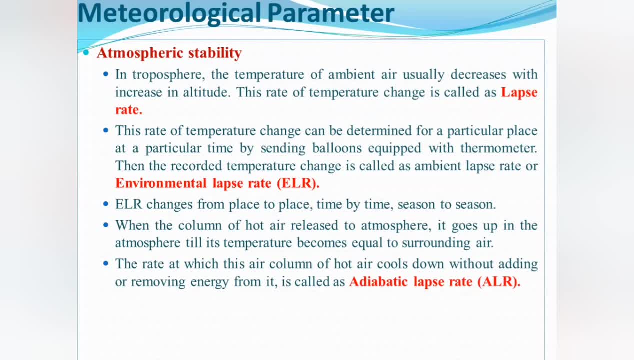 We will leave it in the atmosphere. So, as it goes up, its temperature will be less. The temperature will be less. So how long will it go to the higher altitude Until its temperature and the temperature of the atmosphere is not the same? 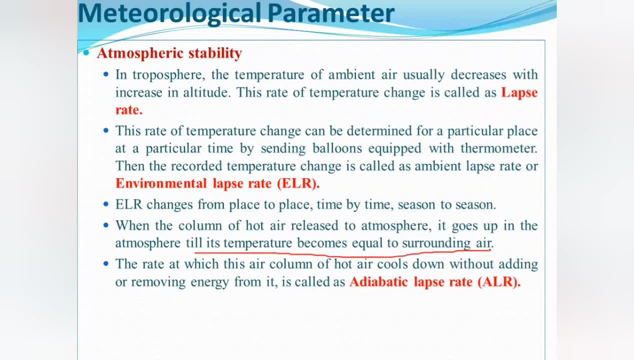 Okay, Now, if this temperature is the same, if the temperature is low, why is the temperature low? That happens. That happens Because its exchange, the exchange of heat, is the exchange of heat from the atmosphere, from the surrounding. Okay. 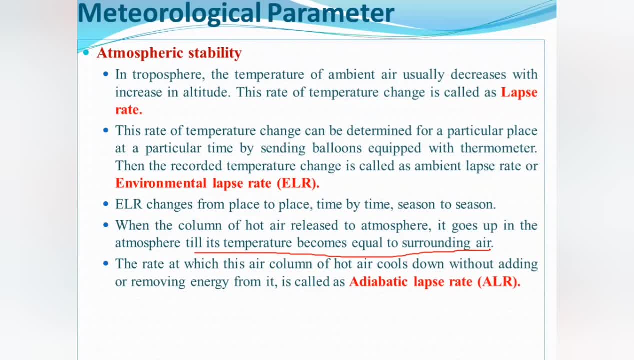 So that is why it is called temperature. If the air in the balloon, the air in the balloon when it goes up, its temperature is decreasing, But its temperature is decreasing, But if its heat exchange or energy exchange is not happening with the environment, then what will we call it? 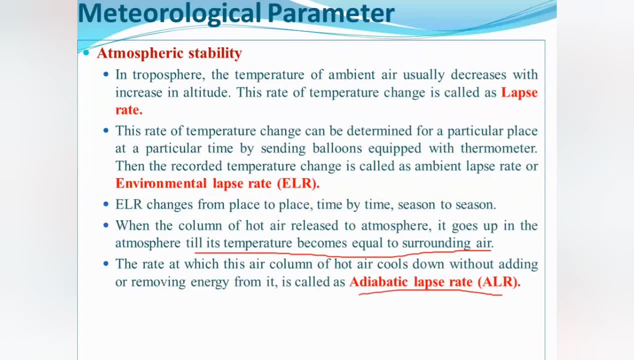 We will call it adiabatic lapse rate. What is adiabatic lapse rate? The rate at which the air column of hot air cools down. The rate at which the air column of hot air, The air column of hot air, cools down without adding or removing energy from it. 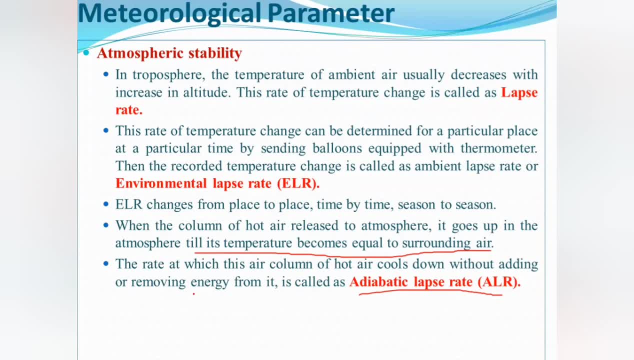 It means that we do not have to add or remove energy from it. It means that without exchanging energy with the surrounding, not exchanging energy from the surrounding or the environment, we will get lapse rate. That lapse rate will be adiabatic lapse rate. 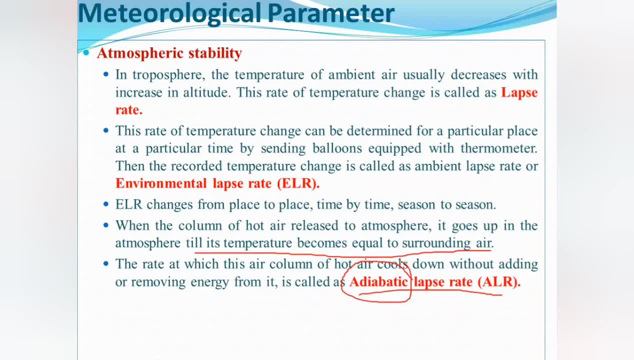 Okay, Now I will give you an example of this. Like thermos, For a long time, the water in the thermos is cold. For a long time, the water is hot. That is why the system inside the thermos does not exchange energy from the external system. 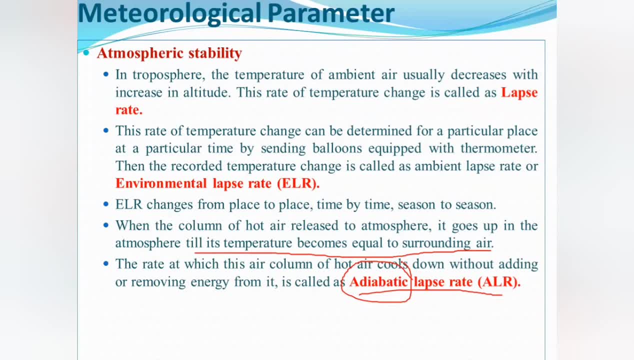 That is why the temperature inside the thermos does not vary. That process is called adiabatic process. Now the meaning of adiabatic here is. the basic meaning of adiabatic is when there is no exchange of heat with the surrounding or the environment. 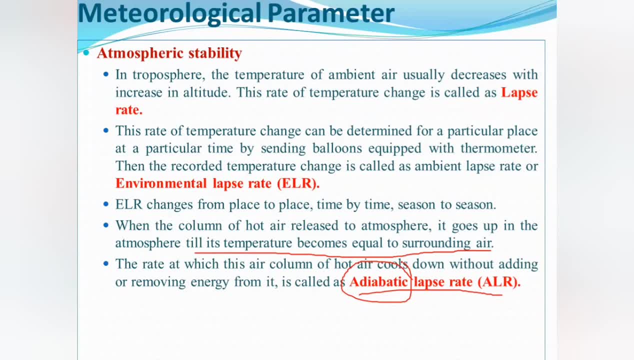 we will call it adiabatic condition And its value is constant Because its value is not going to depend on the atmospheric condition, Because it is not going to depend on the atmospheric condition. That is why it is going to remain the same. 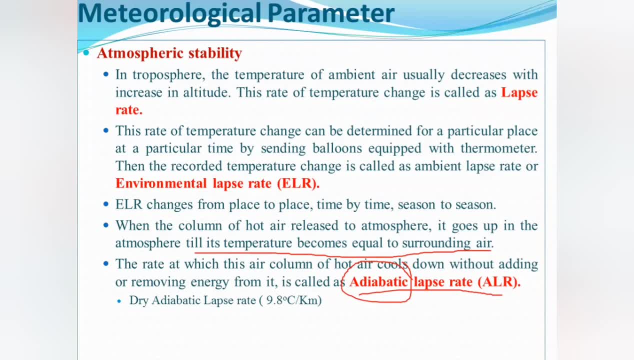 Like if we saw in the morning there was a little bit of atmosphere or a little bit of thunder. in the morning We also sent hot air, So its heat will not be exchanged with the environment. That is why it will not make a difference. 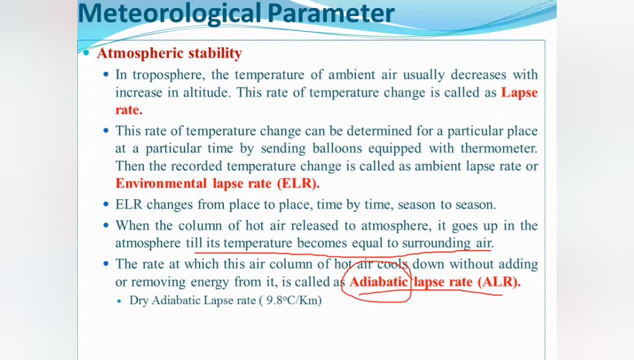 whether it is measured in the morning, in the afternoon or in the evening, Because its heat will not be exchanged with the environment. That is why, throughout the time, throughout the place, throughout the season, the value of adiabatic lapse rate remains the same. 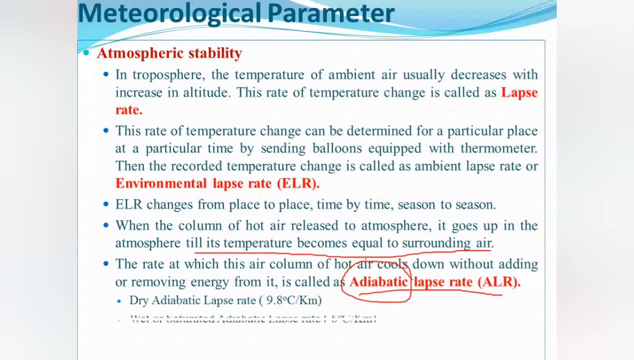 See, it has two types of adiabatic lapse rate. One is dry adiabatic lapse rate and the other is wet adiabatic lapse rate. Now, what is dry adiabatic lapse rate? What is dry adiabatic lapse rate? 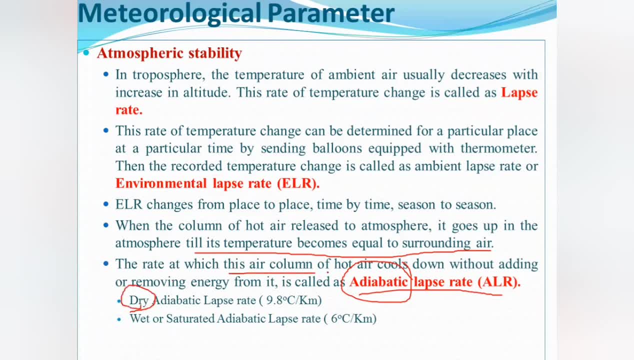 If the air that we have passed, the air that we will pass here, the air that we will pass, if the air in the balloon is dry, completely dry, then the adiabatic lapse rate of that time will be dry adiabatic lapse rate. 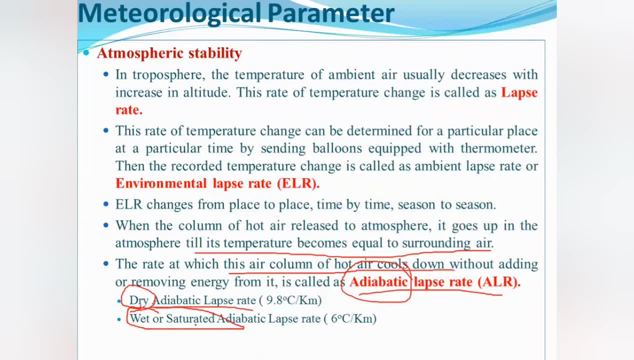 If the air is wet or saturated, then its temperature will be saturated adiabatic lapse rate. Now, what is the value of both of these? The value of both of these is also constant. The value of dry adiabatic lapse rate is 9.8 degrees Celsius per kilometer. 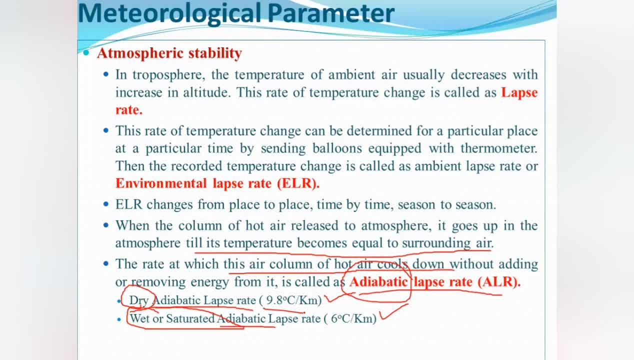 Not per kilometer. If we go one kilometer at a higher altitude, then it will be a decrement of 9.8 degrees Celsius And in wet and saturated adiabatic lapse rate, if we go one kilometer up, then the temperature difference will be 6 degrees Celsius. 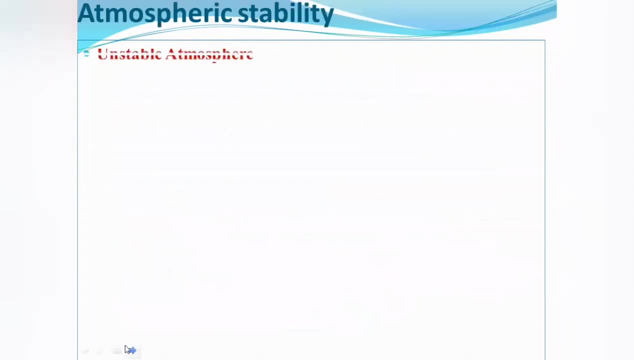 So this was dry adiabatic lapse rate and wet adiabatic lapse rate. Now atmospheric stability. Now, what is atmospheric stability? First of all, we will see the unstable atmosphere. There are three types in total: Stable atmosphere, unstable atmosphere and neutral atmosphere. 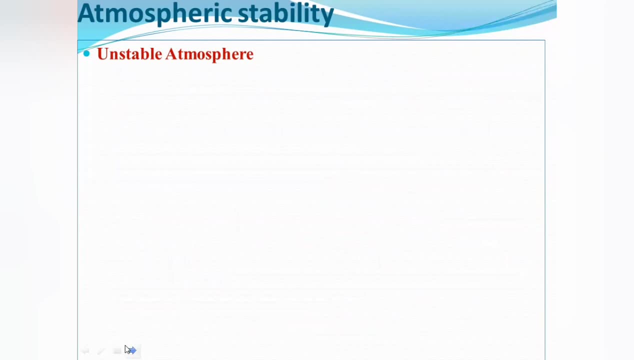 First we will see the unstable atmosphere. When does the unstable atmosphere remain? Atmospheric stability depends on two things, Which two things remain: Environmental lapse rate and adiabatic lapse rate. If the environmental lapse rate is more than the adiabatic lapse rate, 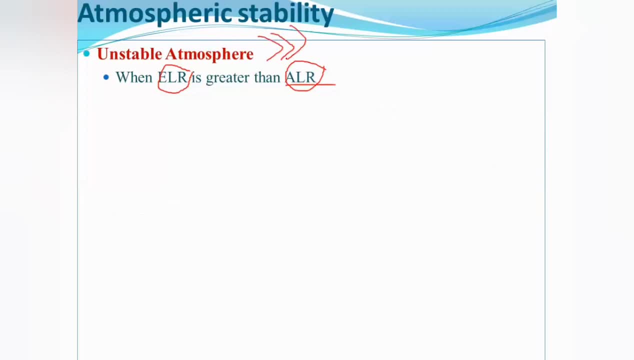 then the atmosphere will remain unstable. When the rate, ie when the rate of cooling of air, is faster than adiabatic lapse rate, then the environmental lapse rate is called as super adiabatic lapse rate And that lapse rate environmental lapse rate. 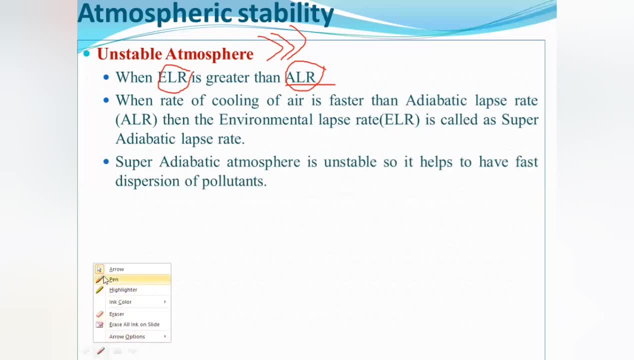 has been categorized again. It will be called super adiabatic lapse rate. When, When the environmental lapse rate is more than the adiabatic lapse rate, Then the super adiabatic atmospheric unstable, So it helps to have faster dispersion of pollutant. 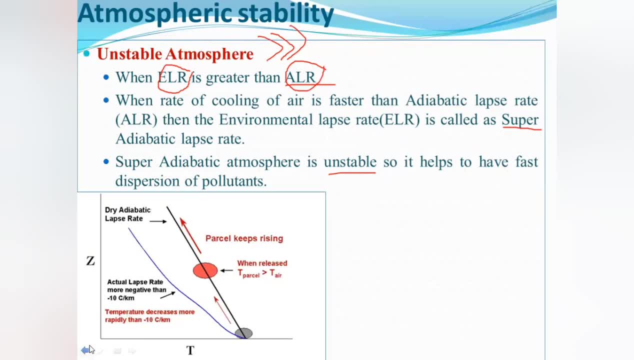 Now let's see how See in this diagram. This is the variation. What is this variation? Adiabatic lapse rate is the constant And the blue line below is the dry adiabatic lapse rate, And the environmental lapse rate is that. 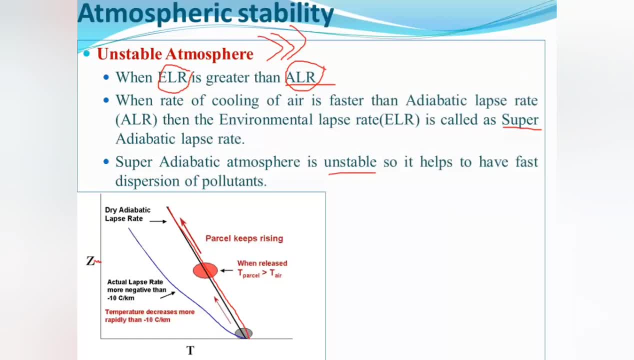 Now here the environmental lapse rate. suppose this is the marking of 1 km. In the 1 km mark of altitude I have extended the marking in 1 km, So for 1 km, when the temperature in the bottom was the same. 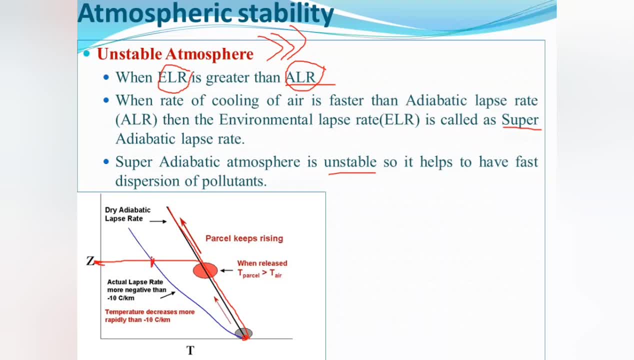 when we went 1 km up. then what will be seen after going up? That the temperature of this particle has decreased more And the temperature of the particle here has decreased less. Now what happens in this? Let me tell you another diagram here. 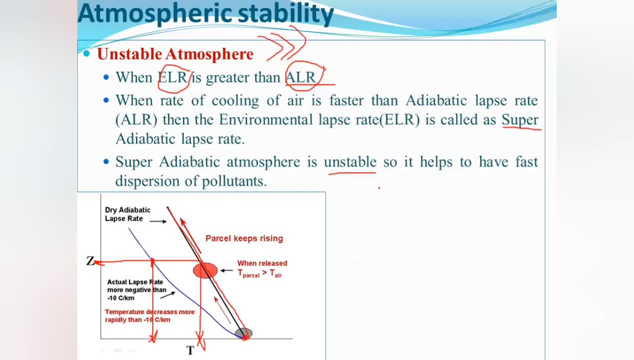 Why is it unstable? Or why is it dispersion? See here Now what happens in the environmental lapse rate, The air parcel that we have placed in the atmosphere. what is its temperature? It stays more. What is its temperature? It stays more. 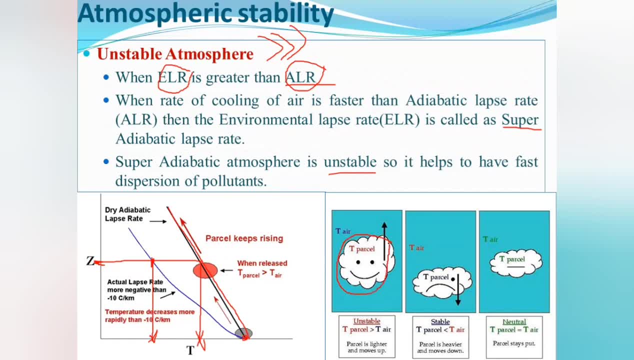 Now what is going to happen? because its temperature stays more? That to maintain its temperature or to bring equilibrium? what will it do? That where the temperature is low, where the temperature is low, it will try to go there. Now suppose its temperature is 25 degrees Celsius. 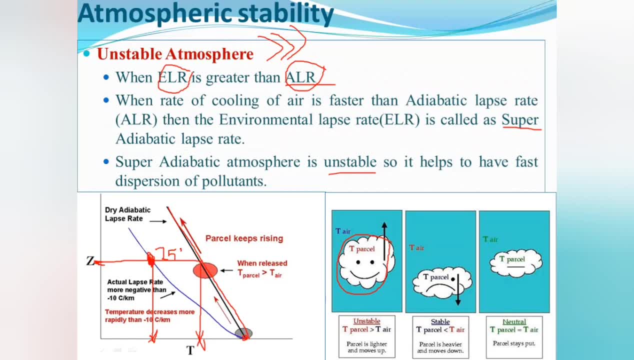 Assume its temperature is 25 degrees Celsius. Now we know that. what happens in daytime? What is the temperature at the higher altitude? It stays low. What is the temperature at the higher altitude? What is the value of the temperature? It is low. 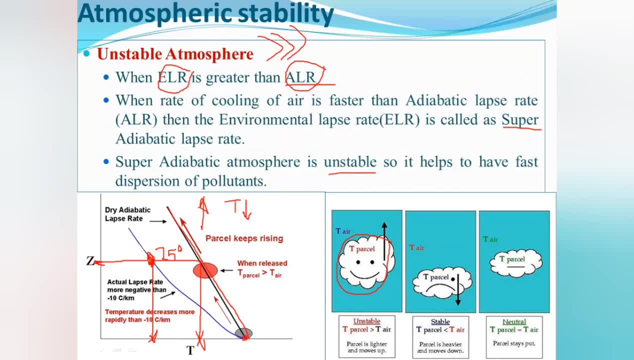 So this particle will not stay here. This particle will go up Because to maintain its temperature or to maintain its equilibrium, it will have to go to the higher altitude. So what will the particle do? The particle will go to the higher altitude. 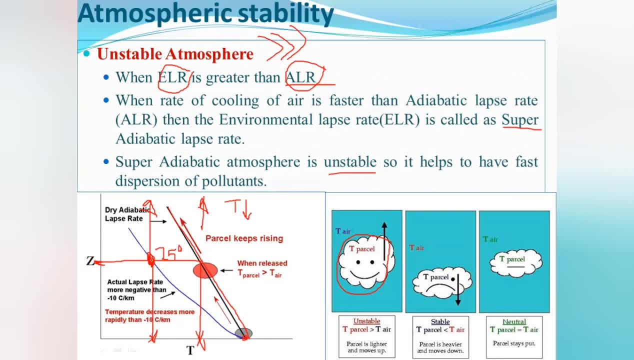 Now the particle or the air parcel will go to the higher altitude. Is the particle stable? No, it is not stable. That is why this condition is called the unstable condition. And the unstable condition is favorable for the environment Because the pollutant or the air parcel will not stay in one place. 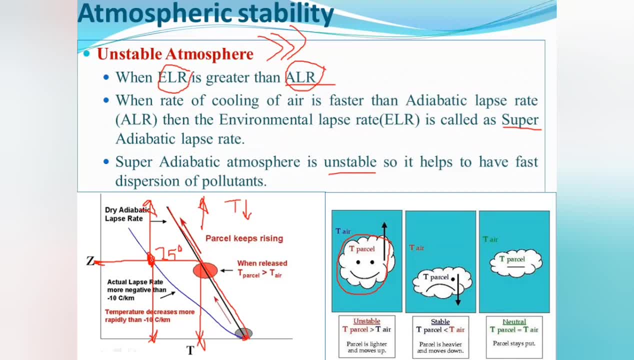 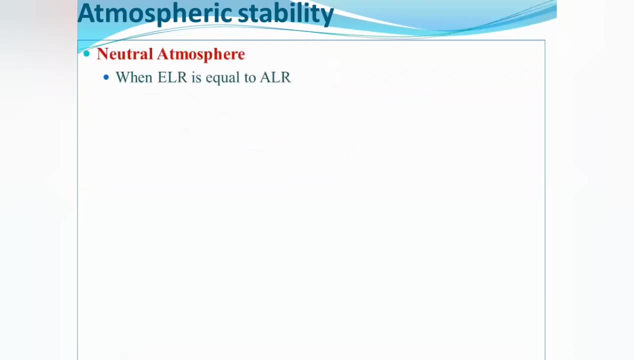 It will be dispersed. If it is dispersed, the concentration will automatically decrease. That is why the unstable atmosphere is favorable for the environment. This is the explanation of the diagram. Let's see the next one: Neutral atmosphere. What is the neutral atmosphere? 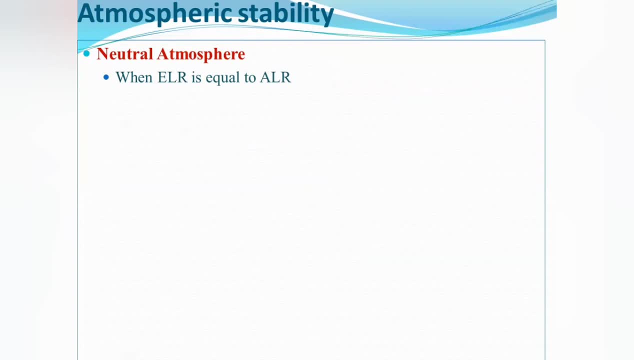 We have to use the same condition of ELR and ALR When ELR is equal to ALR, That is, environmental lapse rate is equal to adiabatic lapse rate. What is the temperature of both? Same When the rate of cooling of air is equal to adiabatic lapse rate. 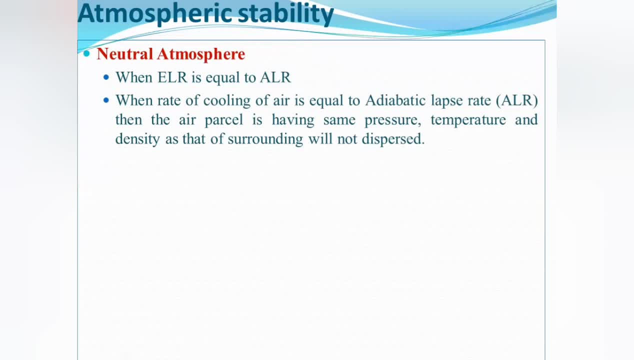 then the air parcel is having same pressure, temperature and density as that of surrounding, will not disperse Because the temperature of the air that we have placed in the air parcel atmosphere, its temperature is already the same as the temperature of the atmosphere And its density is the same. 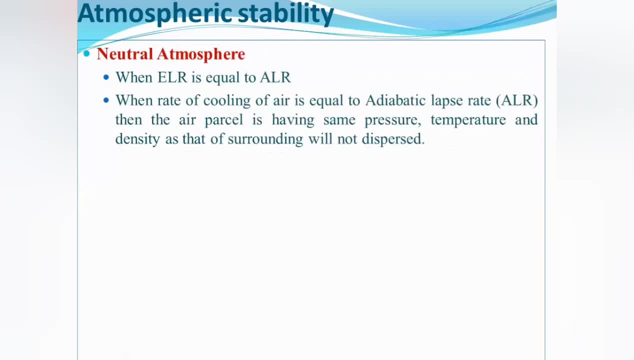 That is why that particle will become uniform with the atmosphere. That is why it will neither go up nor down, nor disperse. Why will it only disperse? Because if the velocity of the wind is more, then only it can be dispersed, That is, according to the turbulence of the wind. 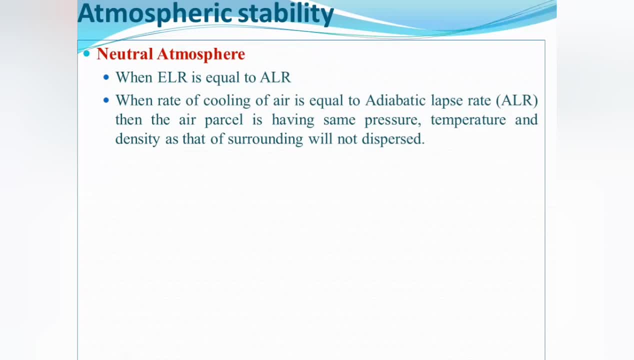 Otherwise it will not disperse. That is why this condition is called neutral condition. When ELR is equal to ALR, Such type of atmosphere is neutral, So pollutant will remain at their position. As I told you, what is this atmosphere? 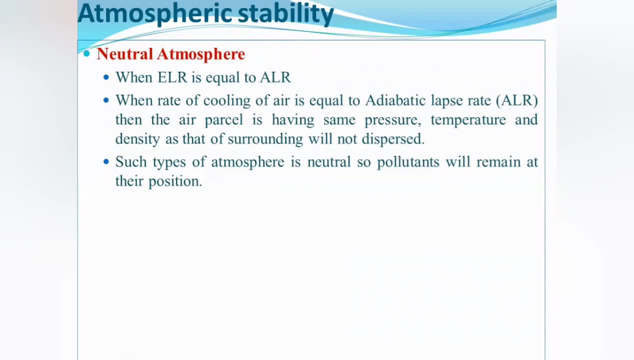 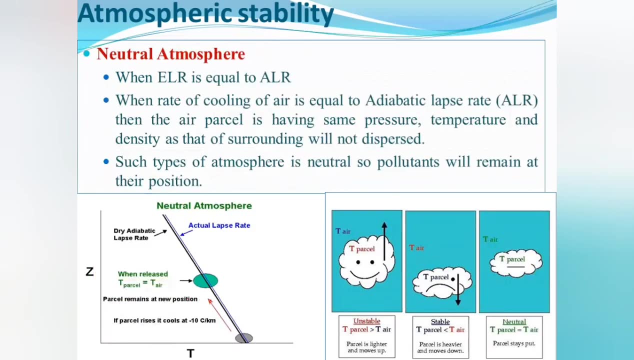 It is a neutral atmosphere, The pollutant here remains there. Then look at the diagram. This graph shows two lines here. One is black and the other is blue. Both lines are the same. Actual lapse rate means environmental lapse rate And dry adiabatic lapse rate. 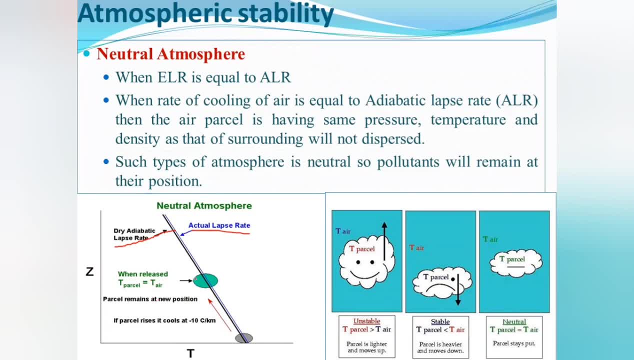 The values of both are the same. That is why the air parcel will remain in the same position, Because both have the same temperature. That is why the air parcel will not move. It will remain there, As you can see in the third diagram. 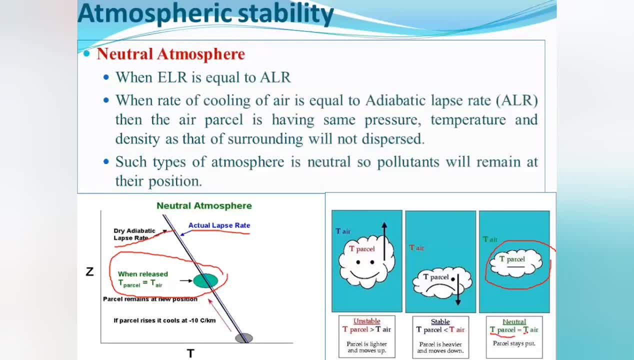 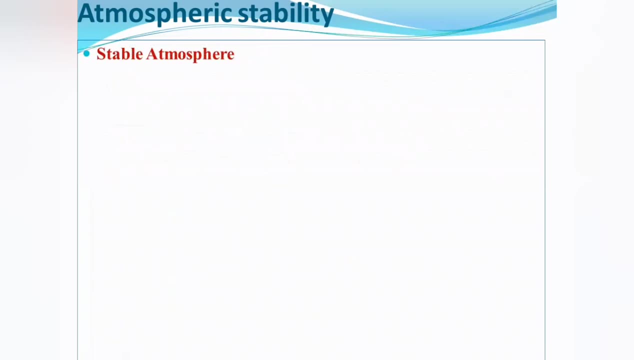 That is, Temperature of parcel is equal to temperature of air. That is why the direction of the particle will not go up or down. This particle will remain stable here. Then third, stable atmosphere. What happens in stable atmosphere When ELR is less than ALR? 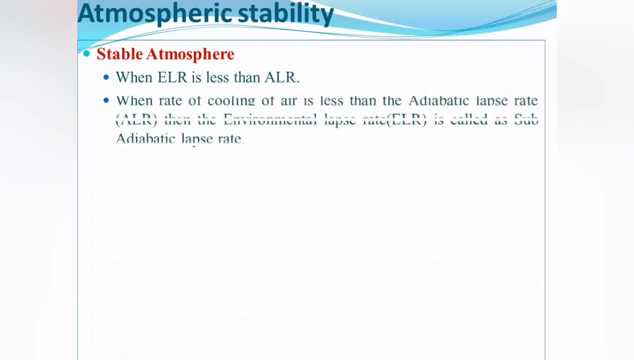 That is, environmental lapse rate is less than adiabatic lapse rate. When the rate of cooling of air is less than the adiabatic lapse rate, Then the environmental lapse rate is called as sub-adiabatic lapse rate. Earlier we saw super adiabatic. 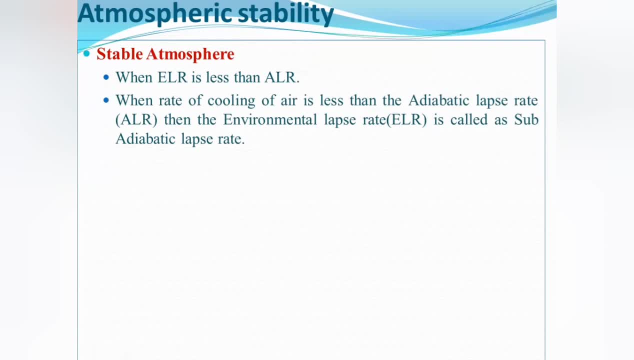 When ELR is greater than ALR, then it is super. When ELR is less than ALR, then it is sub-adiabatic lapse rate. Under this condition, pollutant will not rise. In this condition, pollutant will not rise. 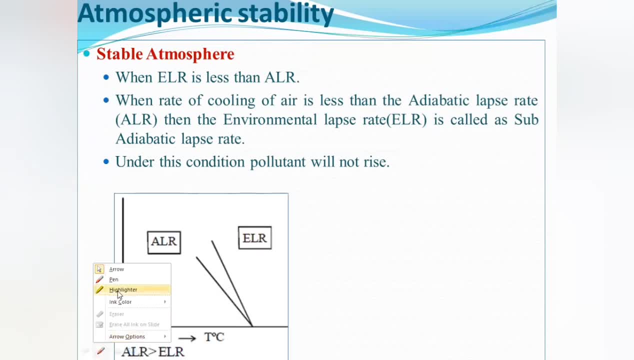 Why it will not rise. I will tell you. Suppose: See Now, this ELR is less than ALR. Suppose here: This is a pollutant. Ok, This is a temperature. Ok. Now If we go to a particular height, 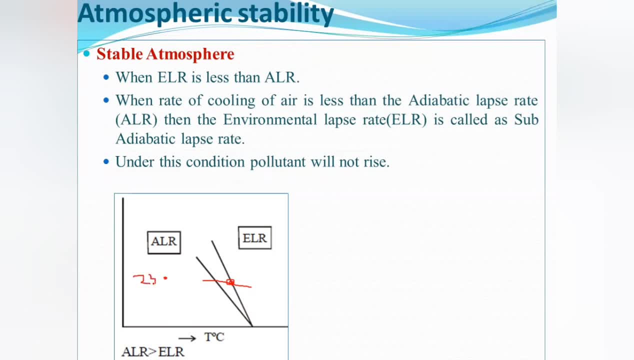 Then, on this particular height, Suppose the temperature is 25 degrees Celsius. Now what will happen? because the ELR is less, As we go up, we will get more temperature. Now, what will happen to this? This is the air, Now its temperature is less than the atmosphere. 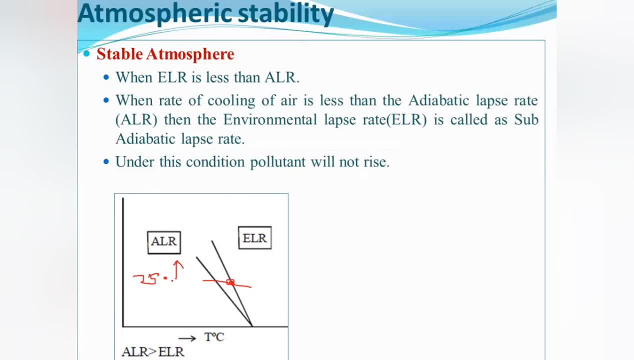 Ok, So what will it do To maintain its equilibrium? this particle will go down. What will this particle be? The particle will go down to maintain its equilibrium. What will we call this Unstable condition? And this unstable condition is highly harmful. 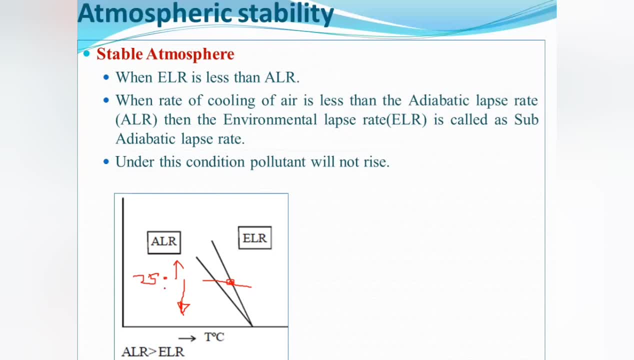 Why? Because where is this particle going? It is going down. It is going down on the ground And on the ground it will come in our contact, It will come in the contact of the environment. That is why this stable condition is very harmful. 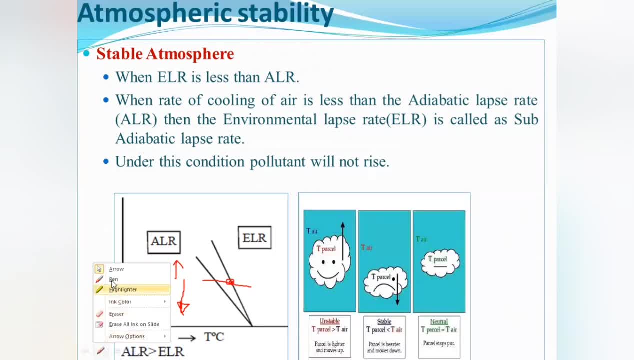 As you can see here in this diagram. Now The parcel, The air parcel, The temperature of the air parcel: The temperature of the air parcel that we have sent. Its temperature is less than the actual temperature of the atmosphere. So what will it do to maintain its equilibrium? 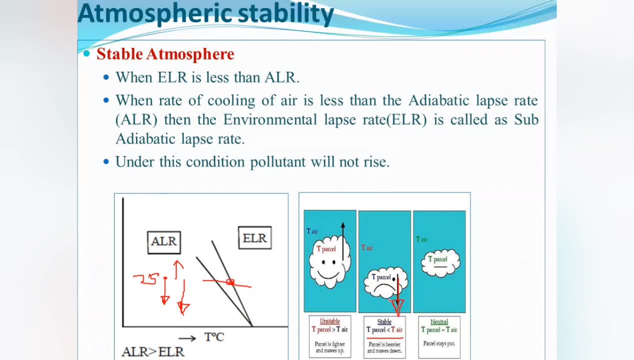 It will go down. And if it goes down, What will happen? Its pollutant contact will come from the environment of the human beings. That is why, Highly, It will develop unfavorable conditions. So keep in mind that the stable atmosphere develops unfavorable conditions. 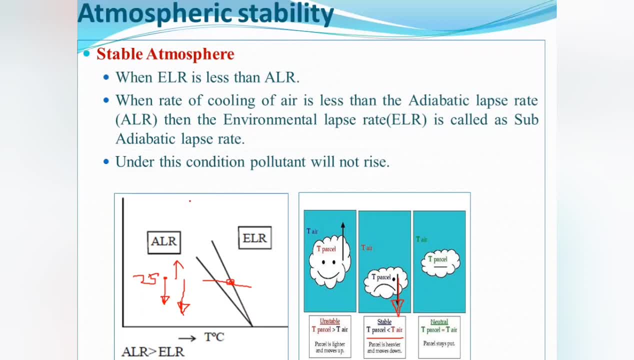 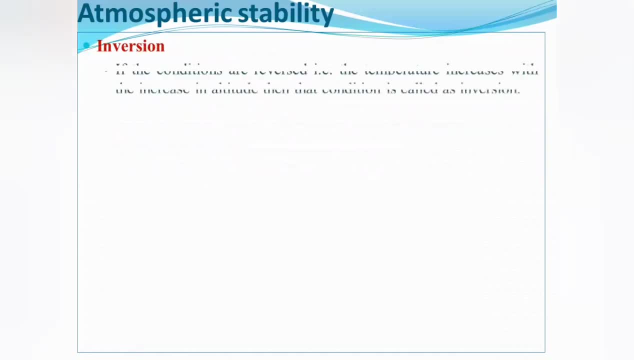 And the unstable atmosphere develops favorable conditions. So this was the stable atmosphere Then. Another temperature variation is inversion, As we have seen. so far As we come to a higher altitude, the temperature decreases. Why does that happen? I told you first. 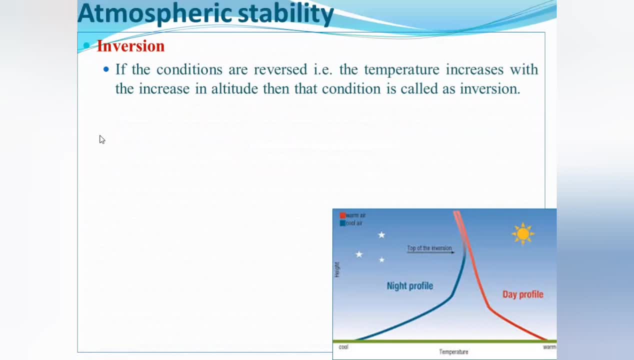 Now what will happen in inversion If the conditions, If the conditions are reversed, Means the condition is reversed, That is, the temperature increases. with the increase in altitude The temperature is increasing. If we increase the altitude, Then that condition is called as inversion. 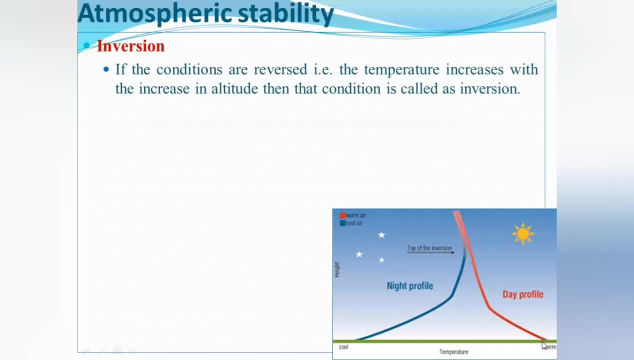 What will that condition call Inversion? Now look at the graph: This line below The line of temperature And the height of the y-axis. Now the red line that you are seeing As we are going to a higher altitude. So what is happening? 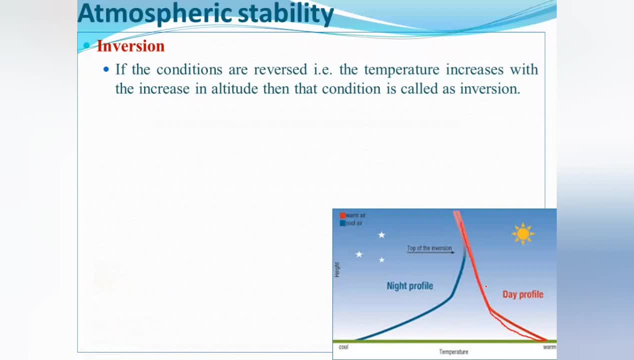 What is happening? The temperature is decreasing. okay, so this is how we see the data in the environmental lab. Now, what happens in the night time is that, as soon as we come to a higher altitude, what is going to happen? The temperature that will increase, will increase the temperature. 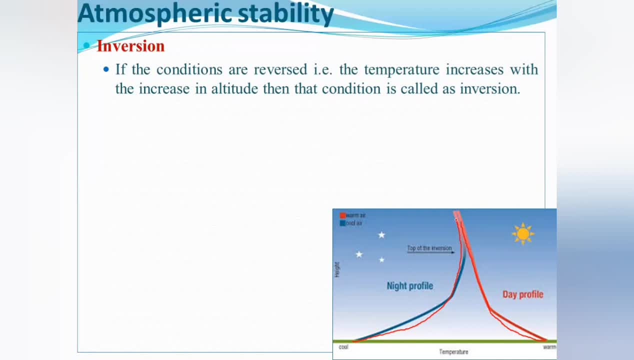 Now this temperature will increase. Why is the temperature going to increase? Let me tell you that, As I told you what happens in daytime, What does the earth do? in daytime, It absorbs heat, And during night time the earth does not get heat because the sun does not reach the earth at night time. 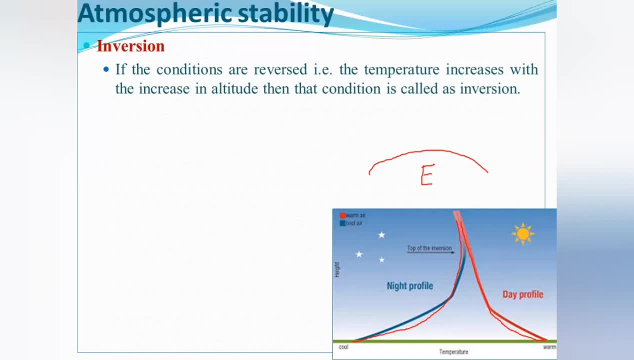 So there is no heat. So what will we do in the night time? What does the earth do in the night? It releases. What does the earth do in the night? It releases heat. So what happens to the earth? Cool down and it gets cold. Keep this in mind From the speed with which any body absorbs heat. 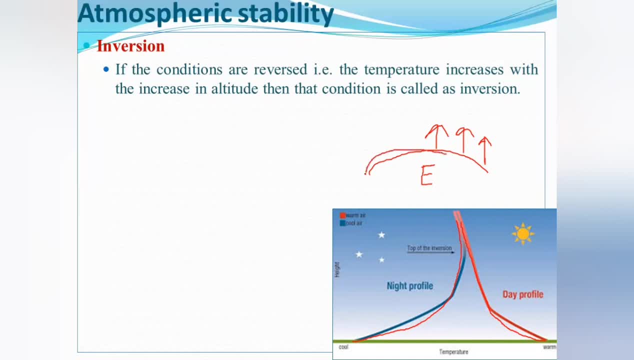 It releases heat faster than it does. So what happens because of this? What happens to the earth? This happens to the earth. The heat is absorbed by the earth. the temperature of the earth will decrease. The temperature of the earth will decrease. 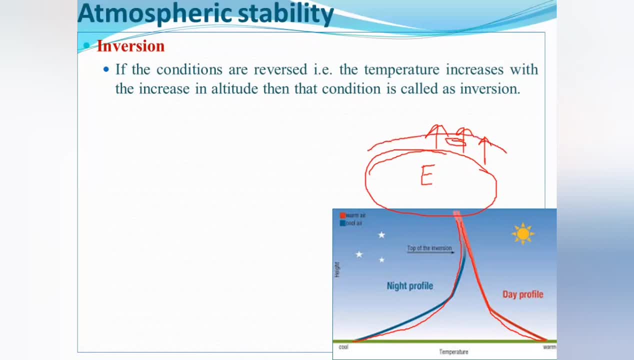 that is, the particles around the earth, the solid particles, sorry gases, particles and atmosphere around the earth will also cool down And as it comes up, how will it stay up? The gases above are less, So the temperature will also. 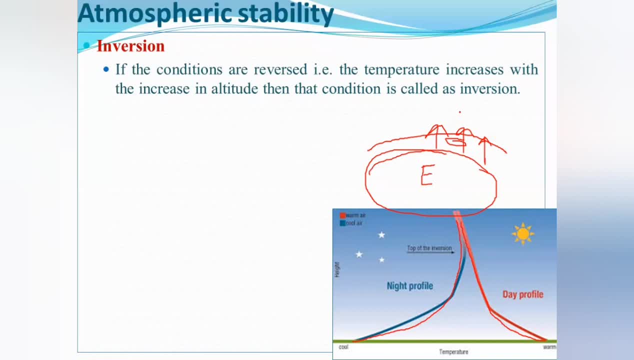 the heat exchange will also decrease. So the temperature variation that is going to happen, that temperature variation will not come as much as in the lower level. What will happen in the lower level? The cold air or the temperature, the heat will release the earth at a higher speed. 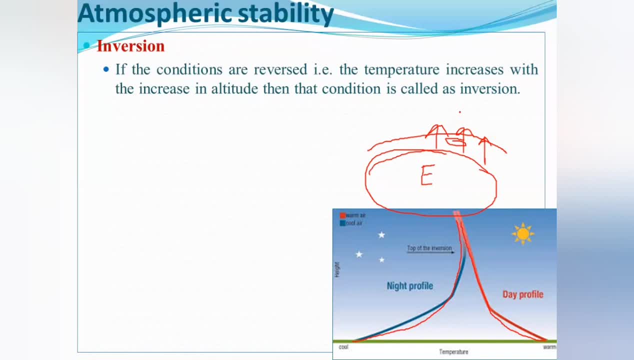 So the temperature in the lower area is less in the night time and in the higher area- sorry, the temperature at the higher altitude is more. What do we do with this condition? Inversion: The lapse rate associated with the inversion is called as negative lapse rate. 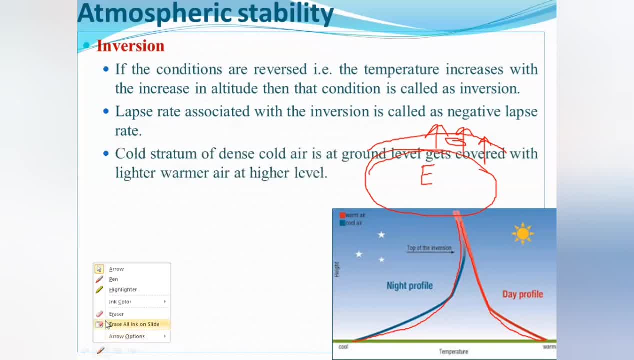 It is also called as negative lapse rate. Then cold stratum of dense cold air is at ground level. Get it, It is covered with lighter, warmer air at higher level. Okay, The cold stratum is at ground level and above that.